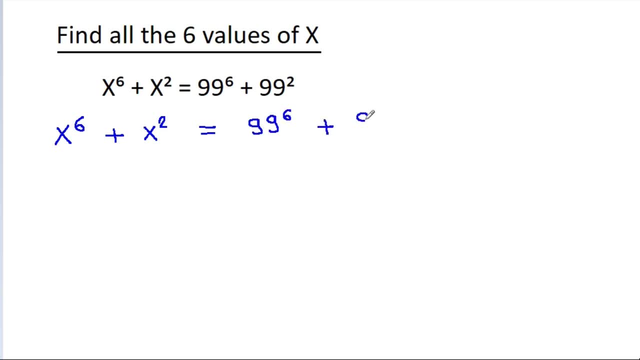 99 power 6 plus 99 power 2.. And it is x power 6 minus 99 power 6 plus x square minus 99 square is equal to 0.. And x power 6 is x square cube Minus 99 power 6 is 99 square cube plus x square. minus 99 square is equal to 0.. 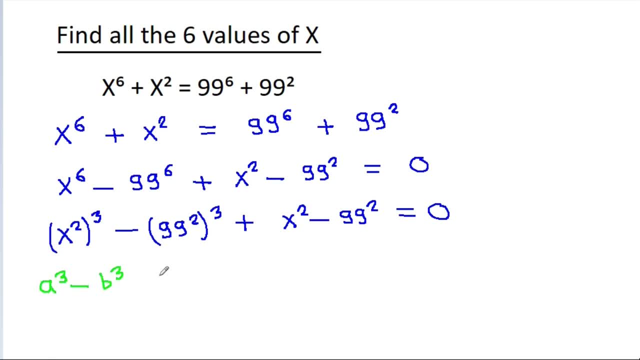 And a cube minus b cube is equal to a minus b times a square plus b square plus ab. So x square cube minus 99 square cube will be equal to x square minus 99 square times x power 4 minus 99 power 4 minus x square times 99 square. 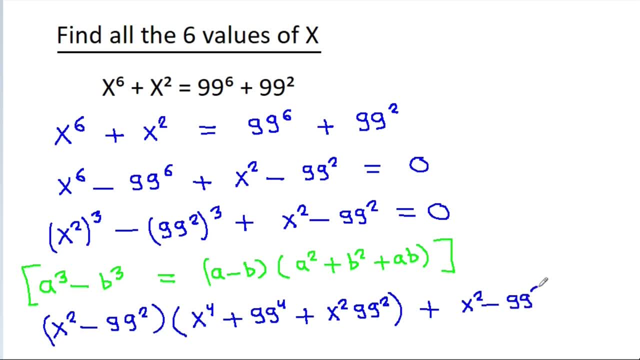 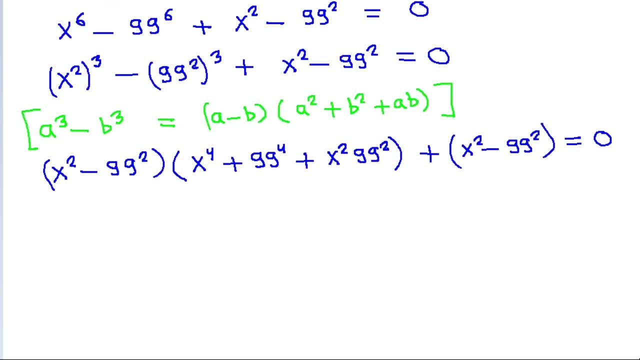 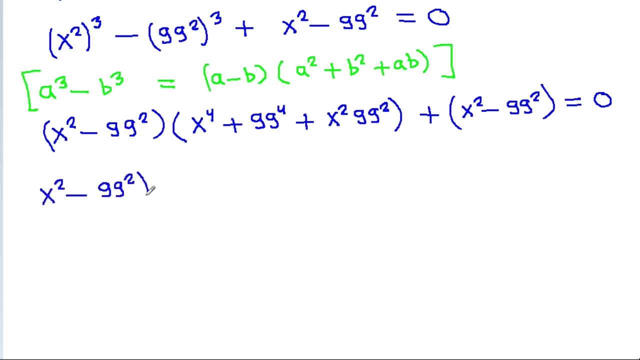 So x power 6 plus x power 2 is equal to 99. power 4 plus x square minus 99 square is equal to 0.. And we can take x square minus 99 square common And we will get x power 4 plus 99 power 4 plus x square 99 square times: x power 4 minus x square 99 square. 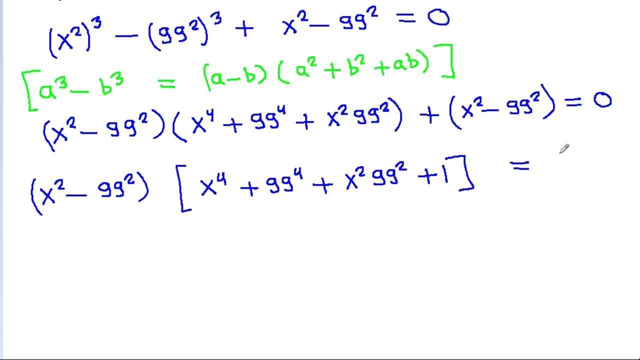 So x power 6 plus x power 2 is equal to 99 square plus x square minus 99 square plus 1 is equal to 0.. And it is x square minus 99 square times: x power 4 minus 99 power 4 plus 99 square. x square minus 1 is equal to 0.. 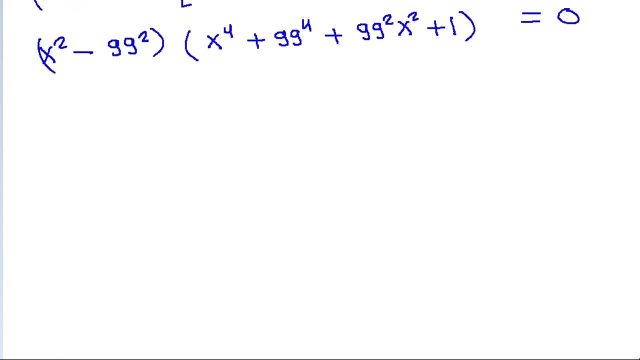 And it is x square minus 99 square times x. power 4 minus 99 power 4 plus 99 square x square minus 1 is equal to 0.. And it is x? square minus 99 square times x. power 4 minus 99. power 4 plus x square minus 1 is equal to 0.. 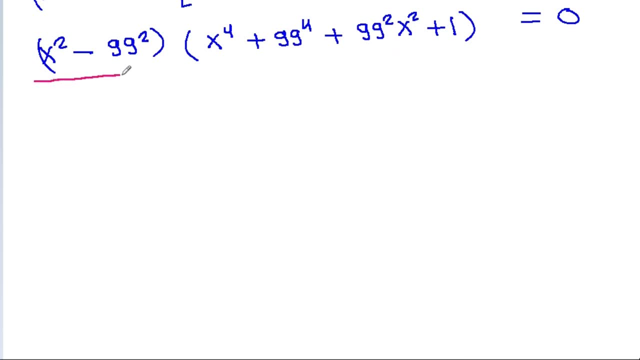 And it is x square minus 99 square times x. power 4 minus 99. power 4 plus x square minus 1 is equal to 0.. If x square minus 99 square is equal to 0, then a square minus b square is a plus b times a minus b. 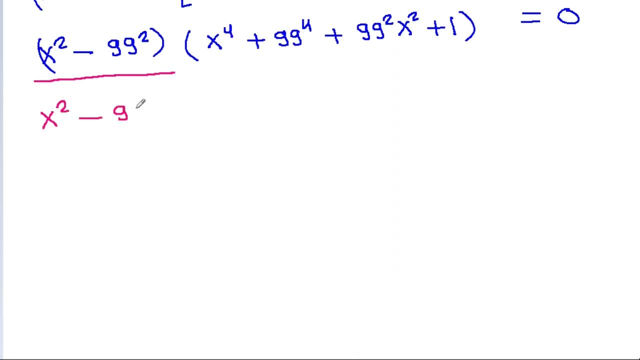 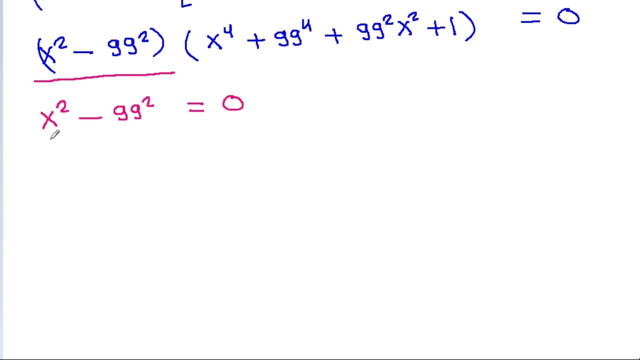 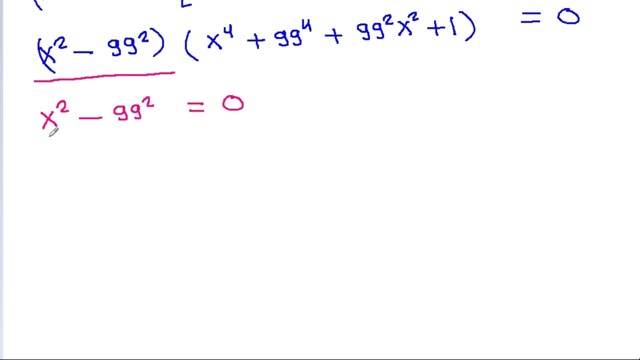 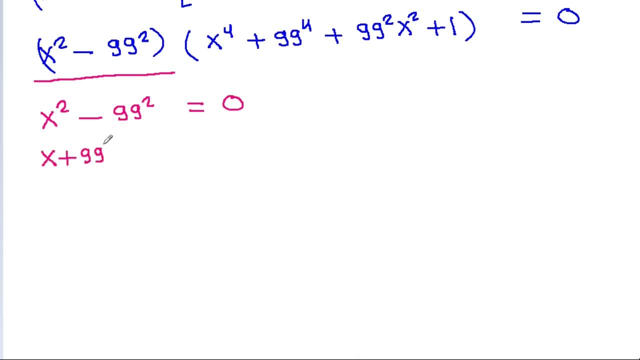 So this will be equal to x plus 99 times x minus 99 is equal to 0.. And from x plus 99 is equal to 0, we will get x is equal to minus 99.. And from x minus 99 is equal to 0,, we will get x is equal to 99. 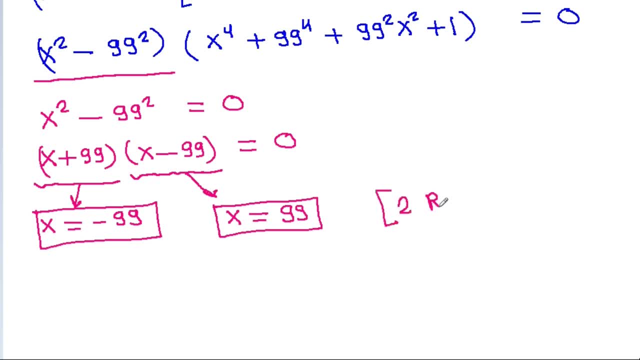 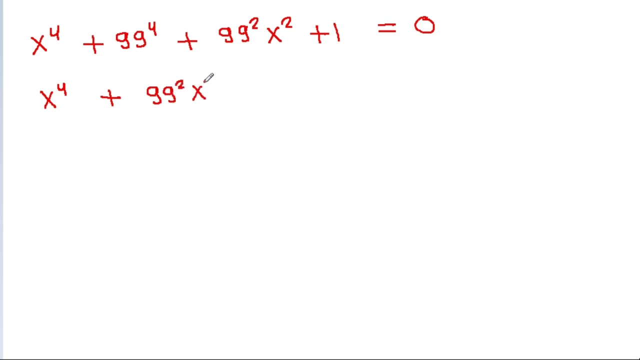 So these are the two real values of x and if this part is 0, if x power 4 minus 99, power 4 minus 99 square x square minus 1 is equal to 0.. Then it is x power 4 minus 99 square x square minus 99. power 4 minus 1 is equal to 0.. 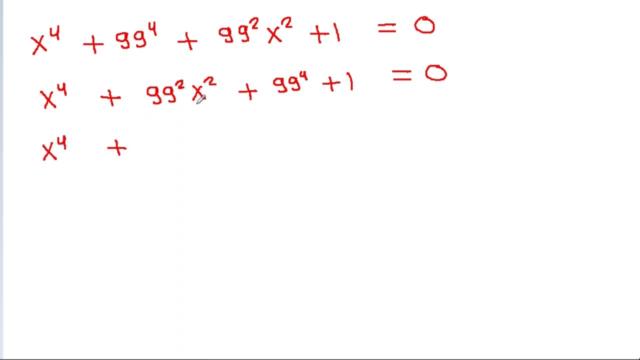 And x power 4.. Plus, And this is 2 times 99 square by 2 times x square plus, and 99 power 4 is 99 x square, x square minus 1 is equal to 0.. And x power 4 is x square, x square plus 2 times. 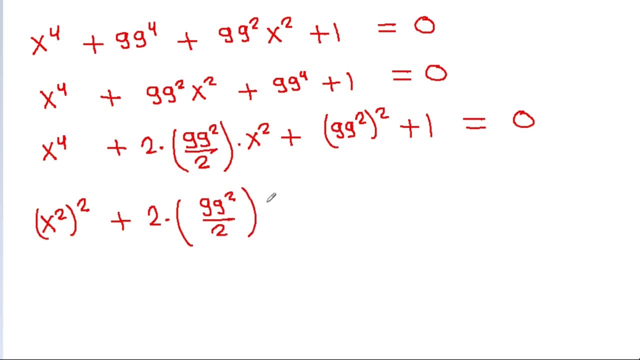 99 x square by 2 times x square plus, and 99 square x square will be 99 x square x square by 4 minus 3, by 4 times 99 x square x square minus 1 is equal to 0.. And it is x square. x square minus 1 is equal to 0.. 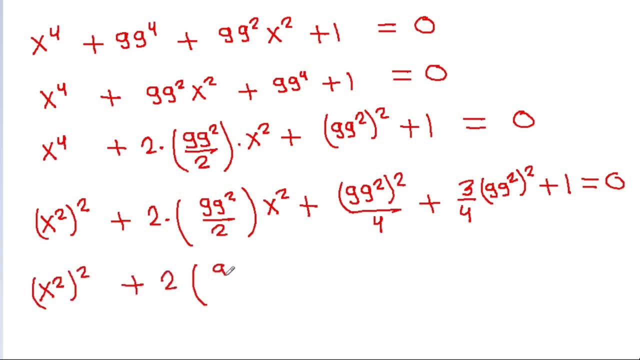 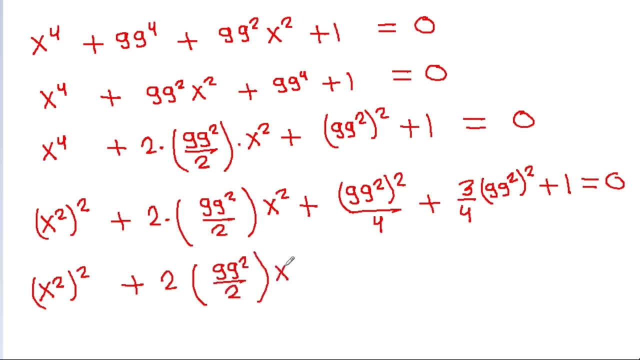 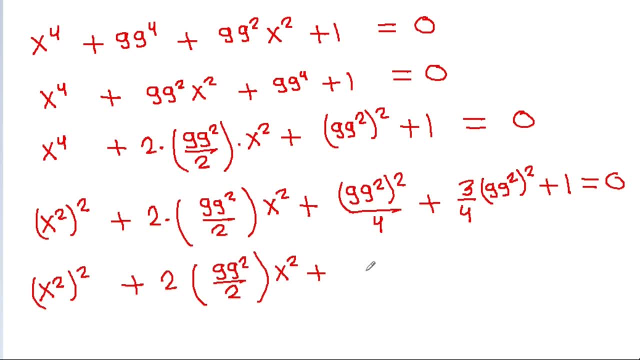 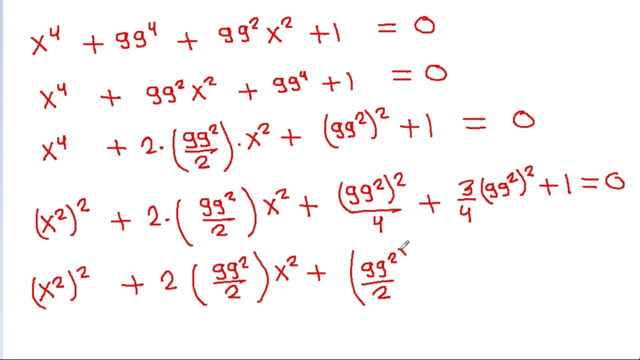 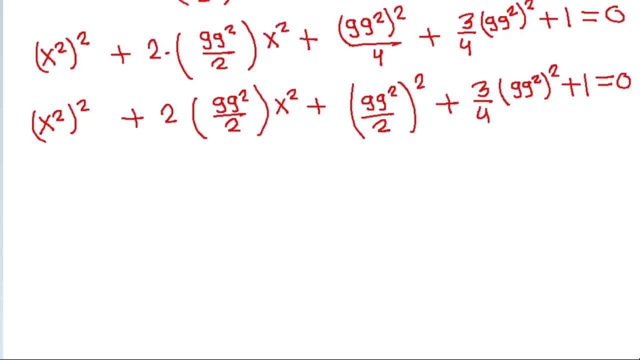 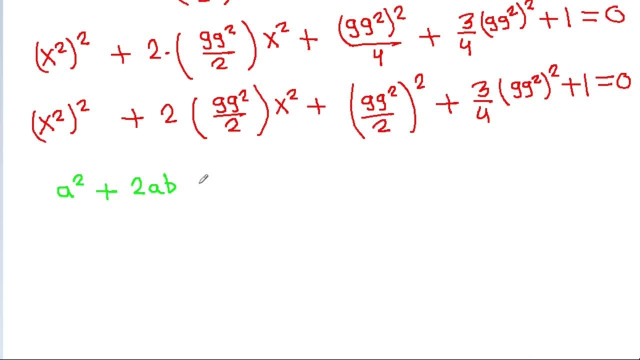 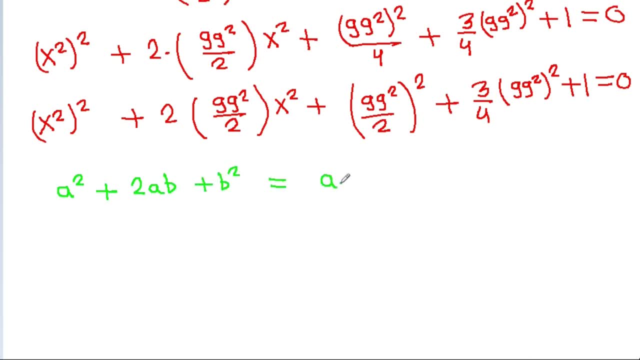 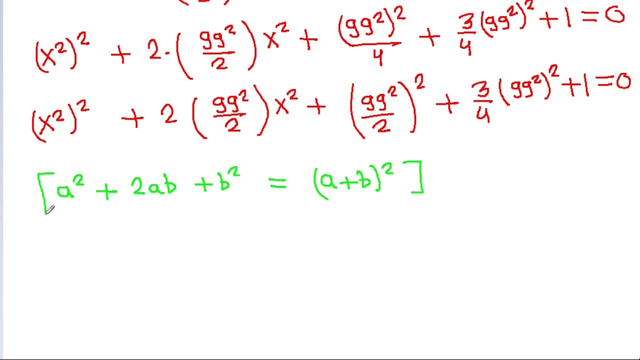 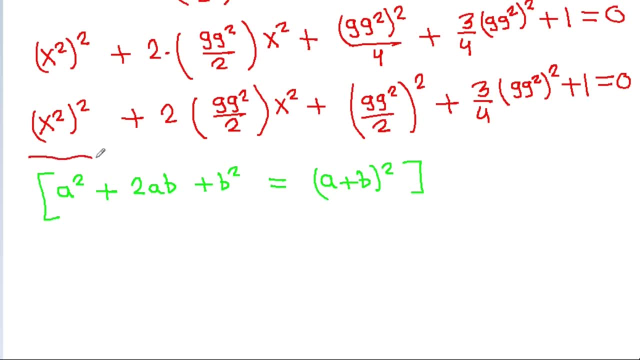 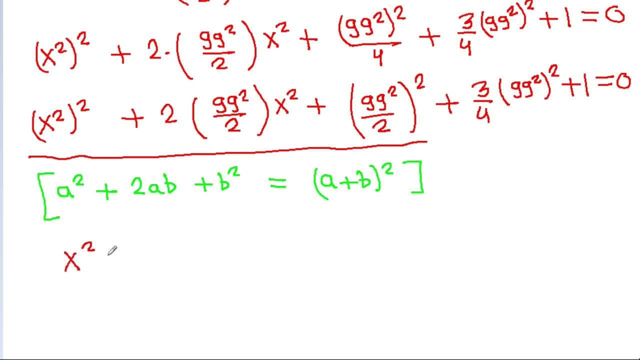 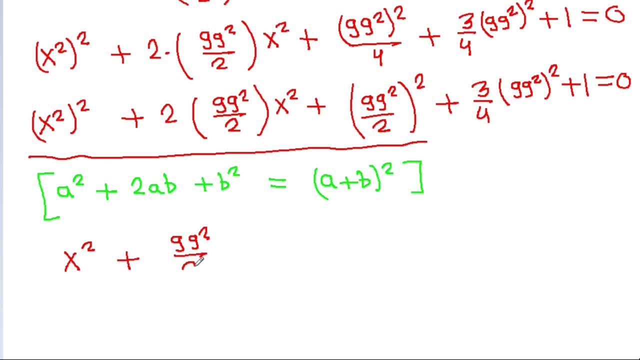 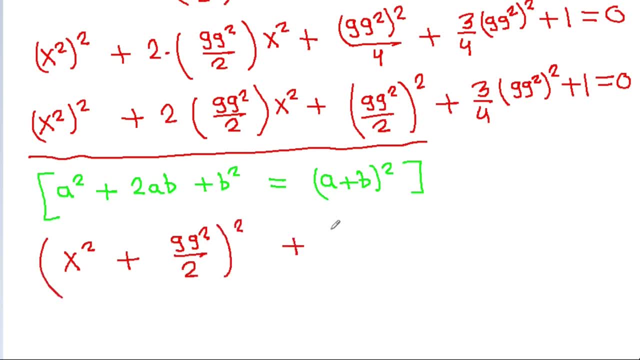 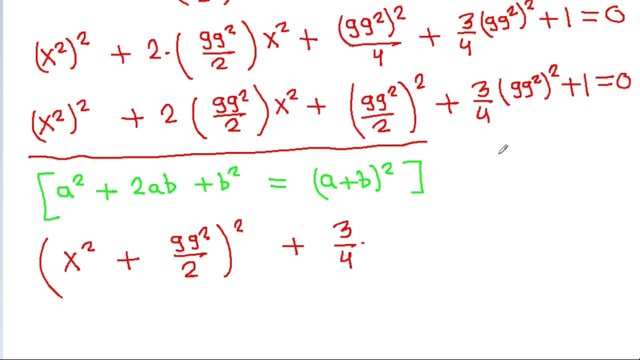 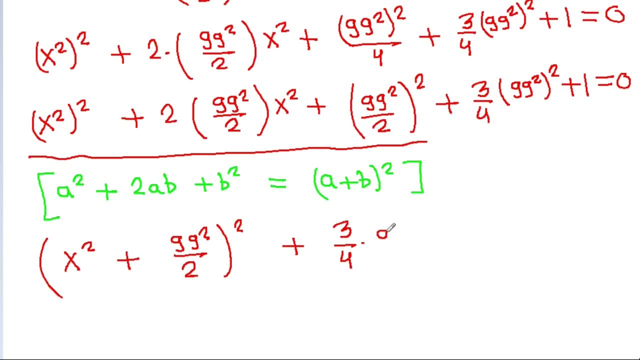 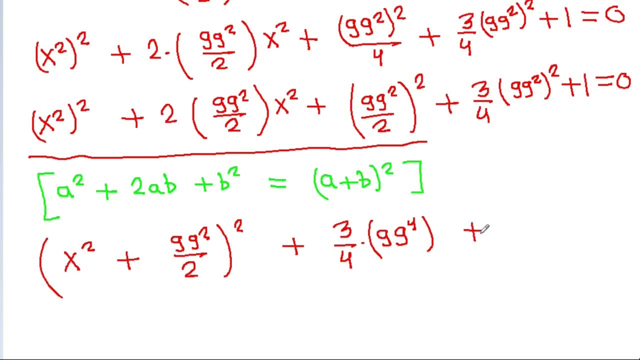 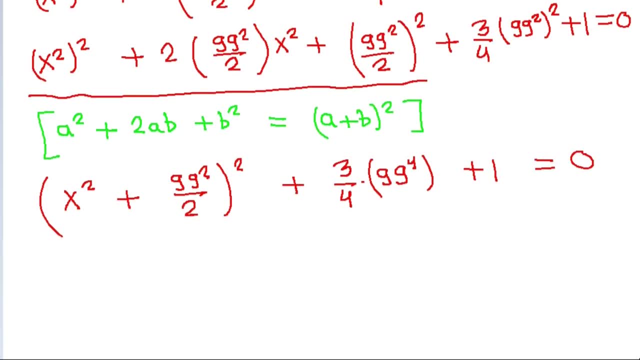 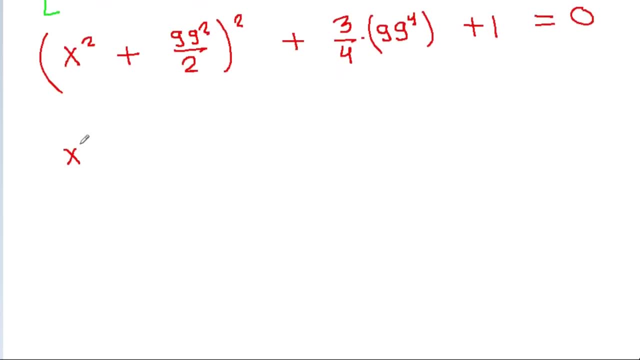 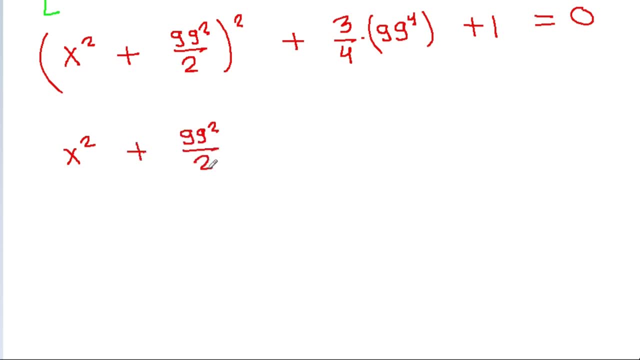 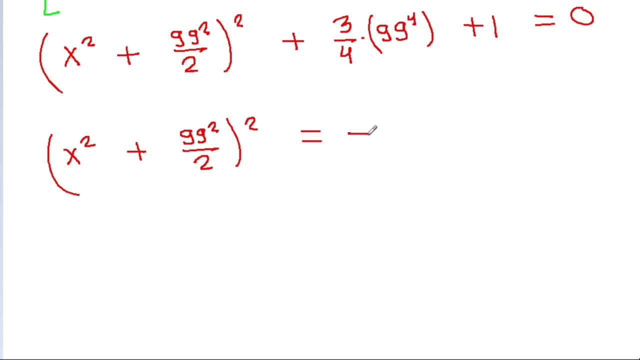 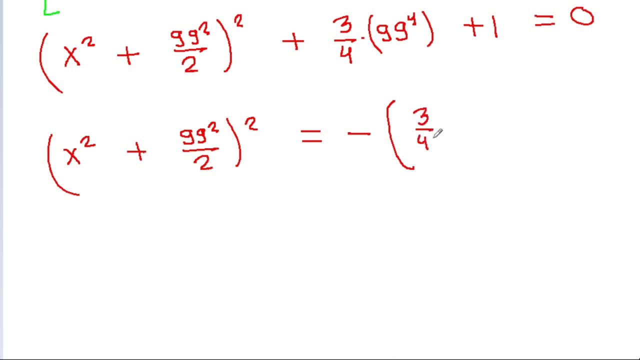 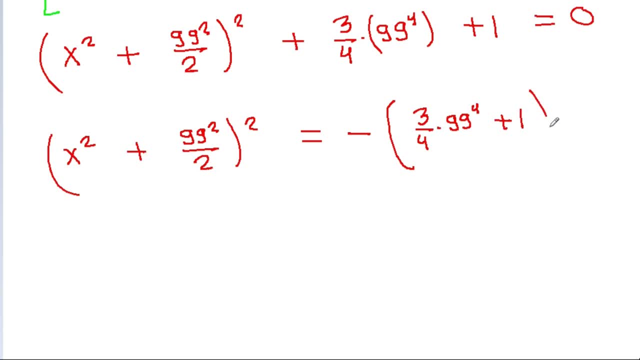 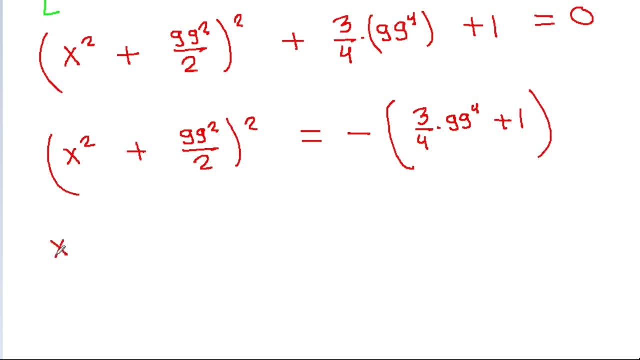 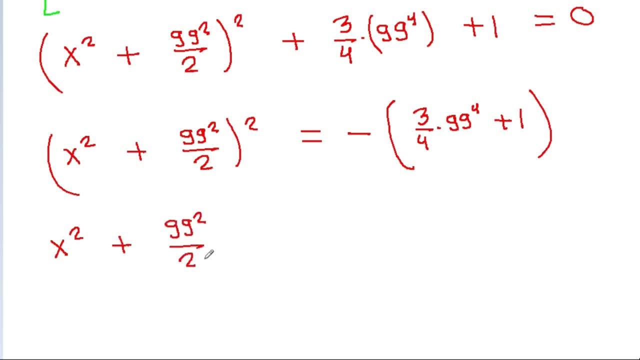 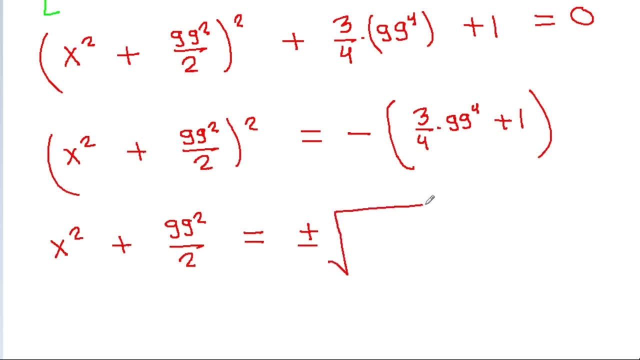 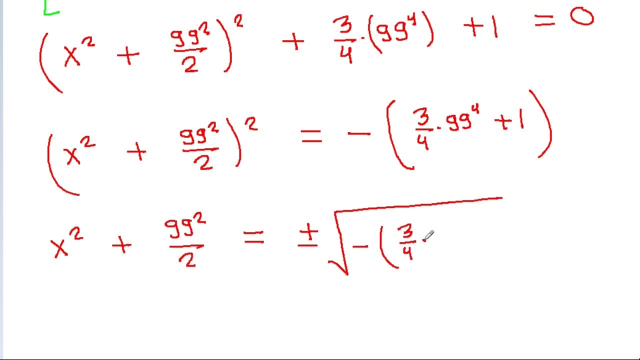 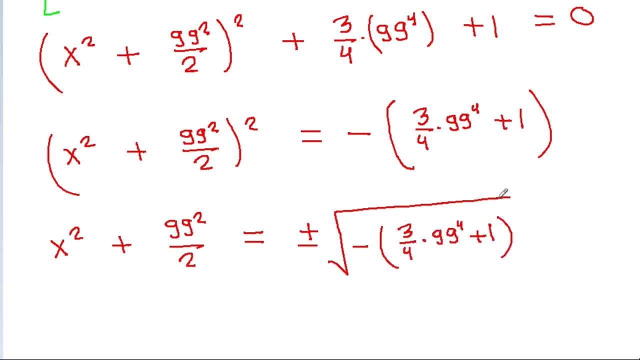 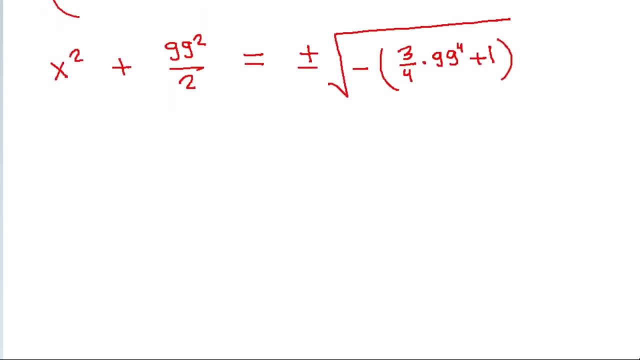 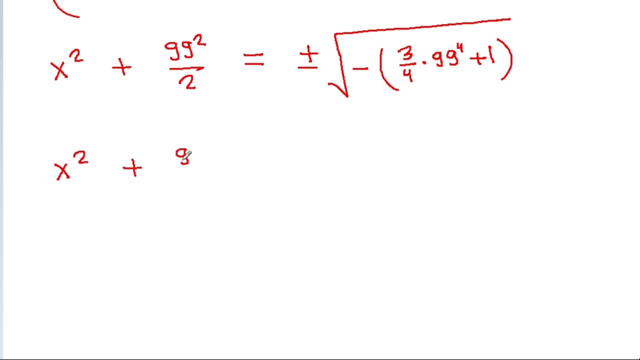 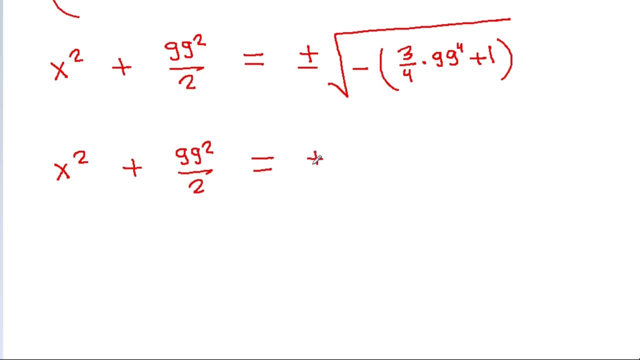 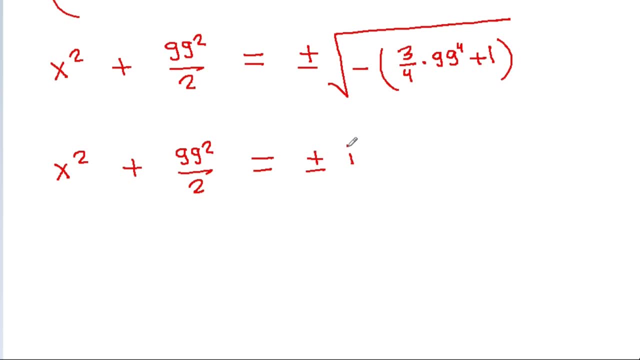 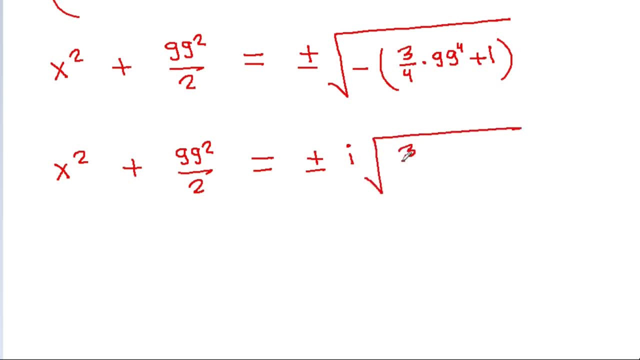 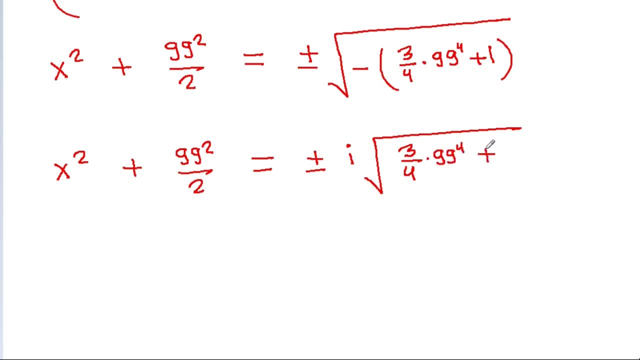 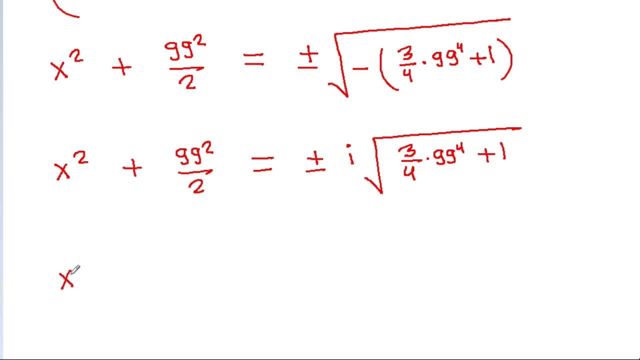 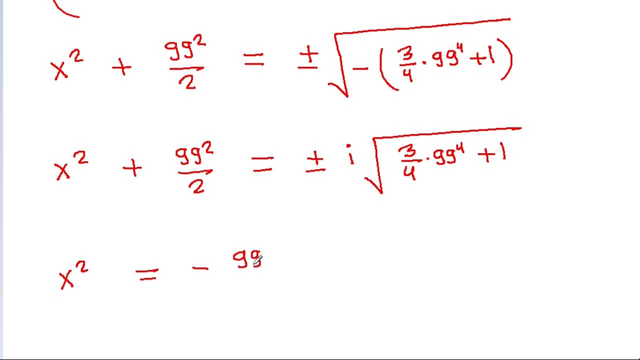 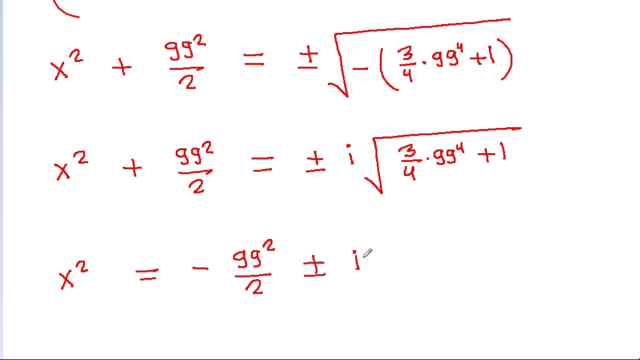 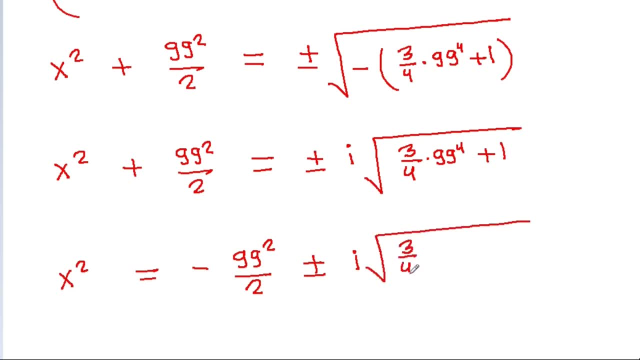 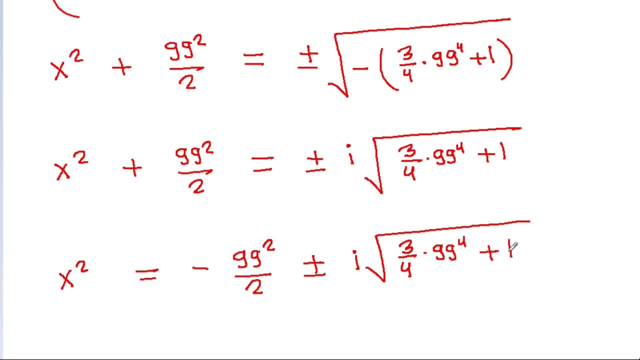 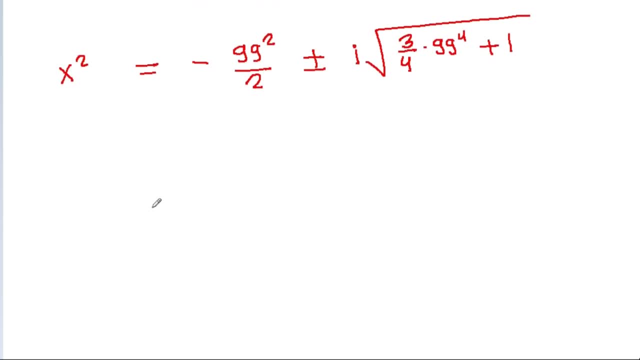 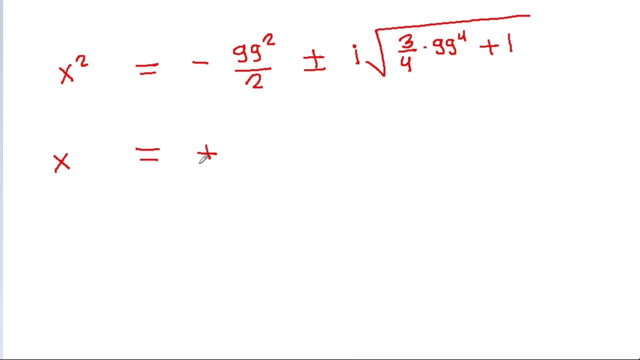 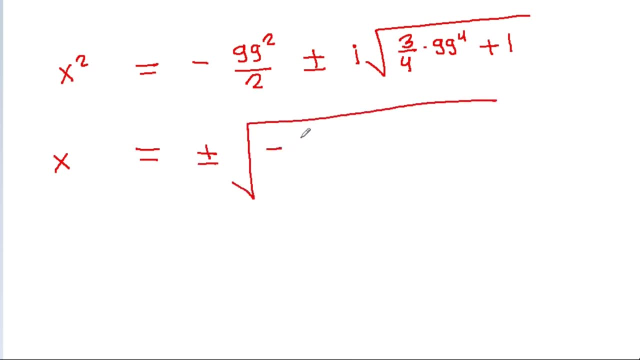 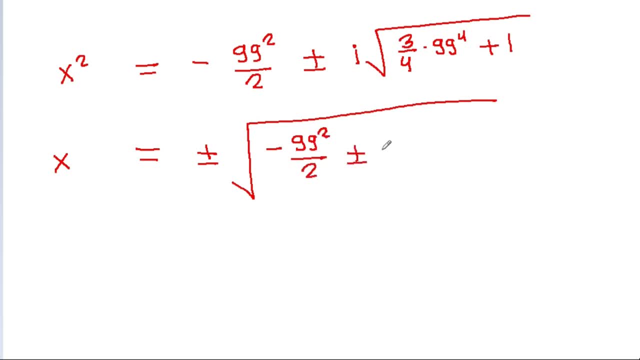 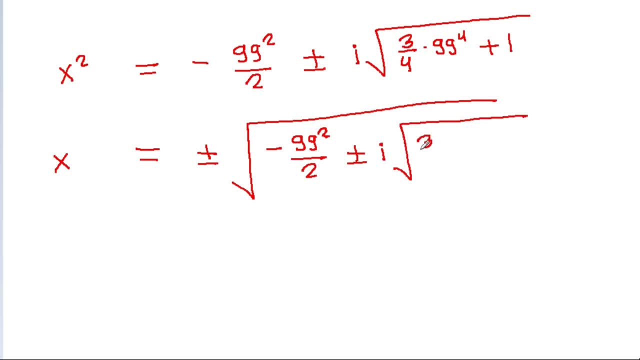 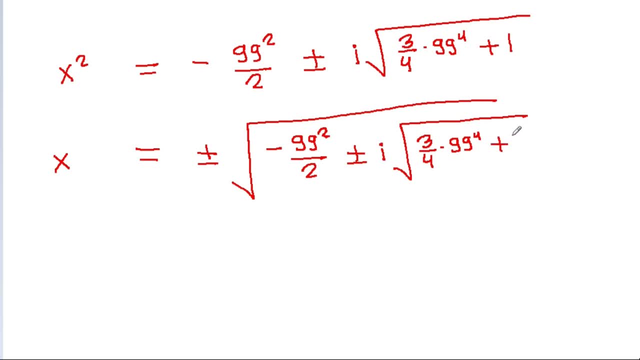 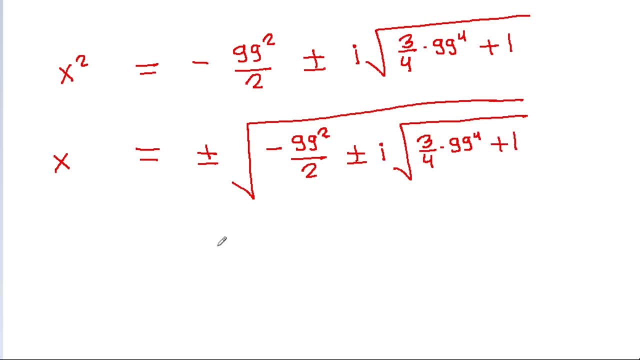 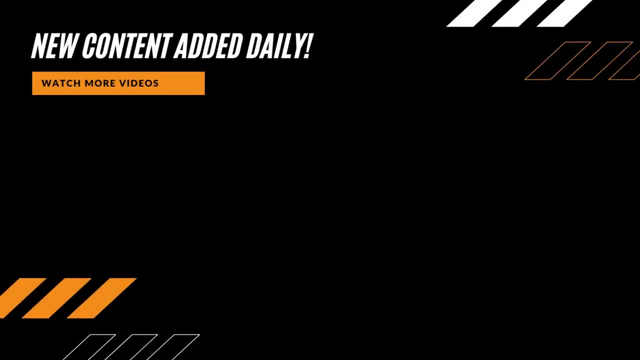 And it is x square. x square minus 1 is equal to 0.. And it is x square: x square minus 1 is equal to 0.. So these are the four complex values of x.